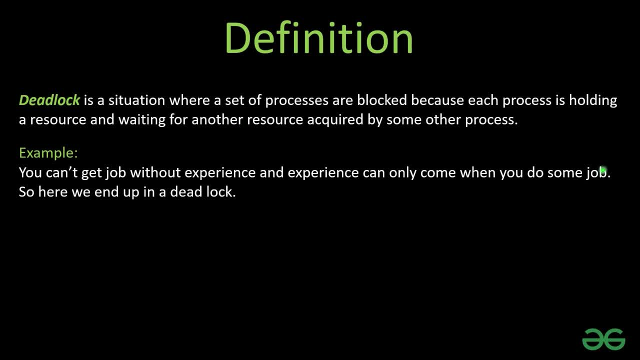 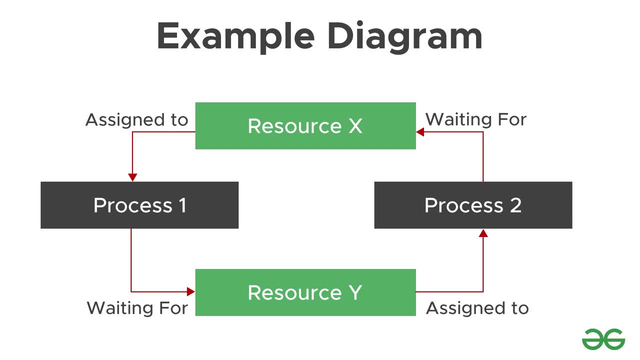 resource acquired by some other process. Let us understand it with the help of an example. So, in this example, process one is waiting for resource Y, but it is assigned to process two. Process two is not getting completed because it requires resource X, which is assigned. 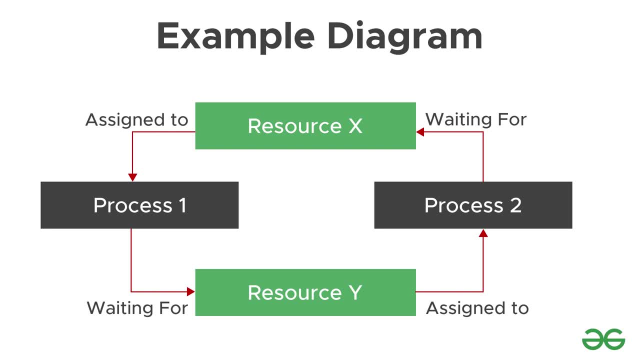 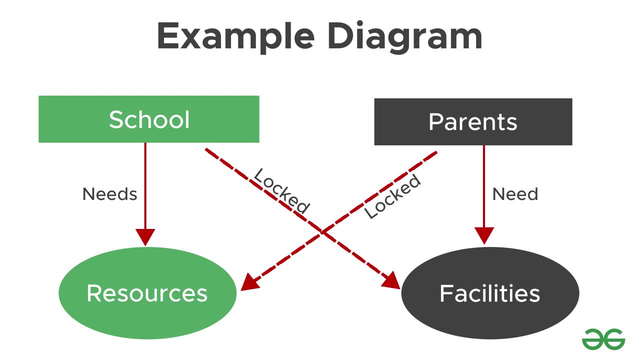 to process one Ending up in a deadlock situation. Let's understand deadlock with one more real life example of a wrongly managed school. The school never performs good in board exams. Almost all the students get failed. When the principal is asked why, his straightforward answer is: 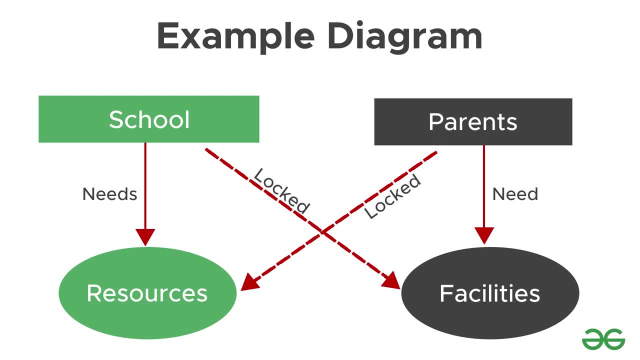 that teachers doesn't teach well. When the teachers were asked about why the students were getting failed, they said that they were not given their wages. Then again, when the principal was asked why they are not giving the wages, The principal says that parents don't pay the fees and he does not have the funds to 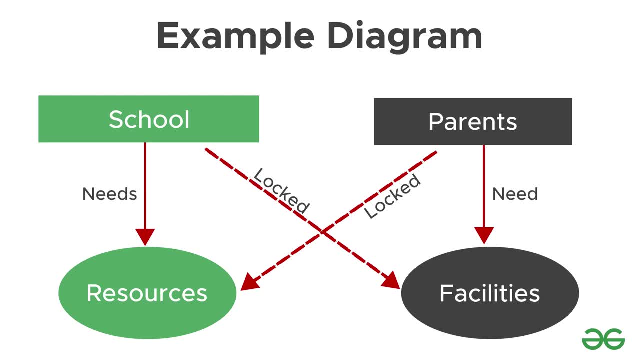 give the pay to the teachers. The parents give the reason that school does not provide enough facilities. But obviously principal cannot provide facilities unless the fees is paid, which is depicted in this diagram, And parents are not ready to pay the fees until facilities are enhanced in the school. So here we end up in a deadlock situation. 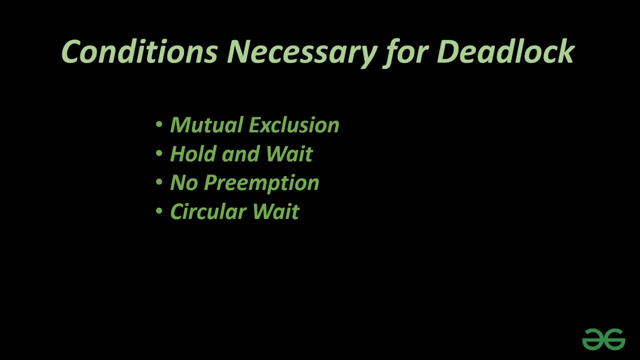 and there is not much we can do for the school. In the previous example we saw a deadlock between only two processes, namely school and parents, But a real operating system deadlock can be complex and it usually involves multiple processes and resources. So now we are going. 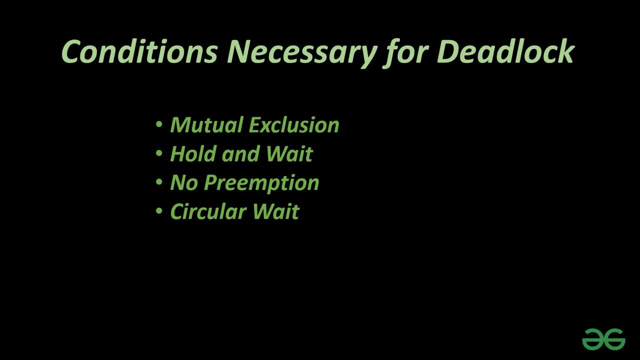 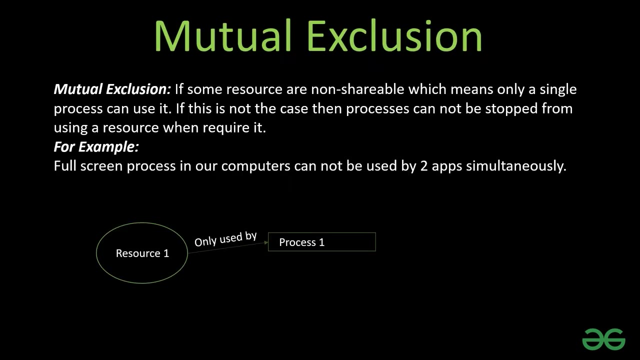 to study four necessary conditions for a deadlock to happen. So they are: mutual exclusion, hold and wait, no preemption and circular wait. Let's see them all one by one. So let's understand mutual exclusion First. some resources are non-shareable, which means that only a single process can. 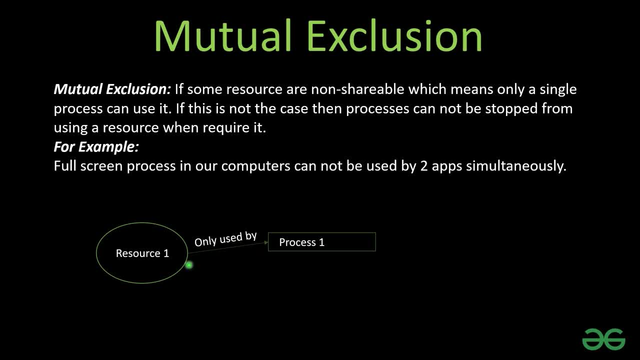 use it. For example, here process one can use resource one and no other process can use resource one. If this is not the case, then process cannot be stopped from using a resource when they require it. For example, full screen processes in our computer cannot.